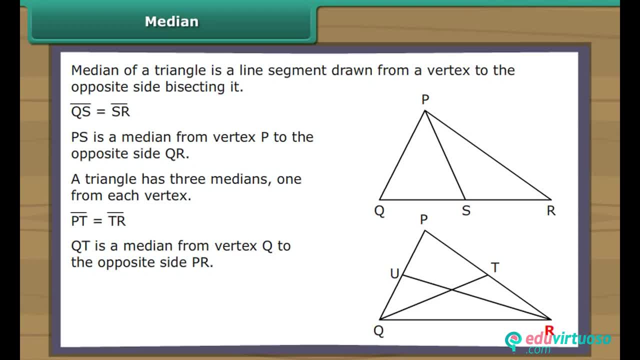 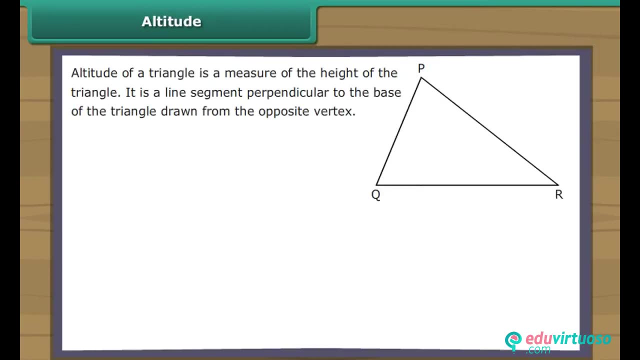 We draw one more line segment from R to cut Q-P into two equal halves at point U. Therefore R-U is a median from vertex R to the opposite side, Q-P Altitude. Altitude of a triangle is a measure of the height of the triangle. 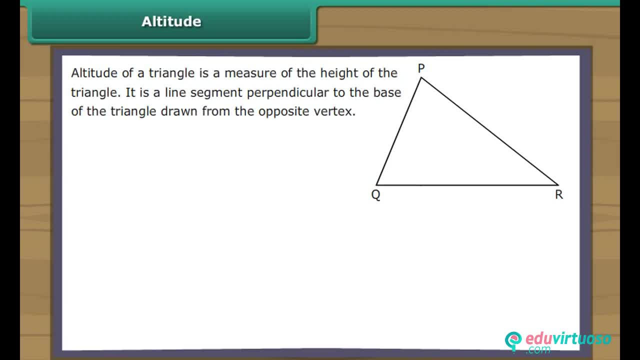 It is a line segment perpendicular to the base of the triangle drawn from the opposite vertex. In the figure line, segment P-S is a perpendicular to the base of the triangle drawn from the opposite vertex. It is a line segment perpendicular, drawn from the vertex P, to the base Q-R. 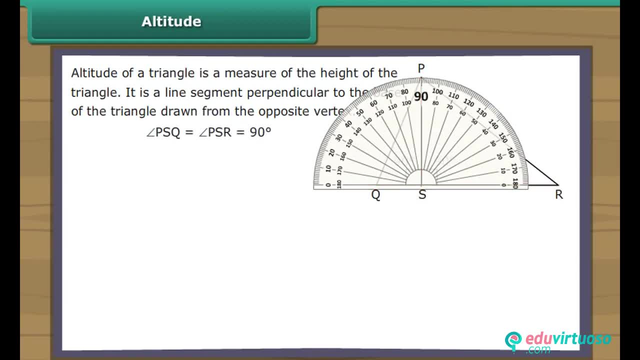 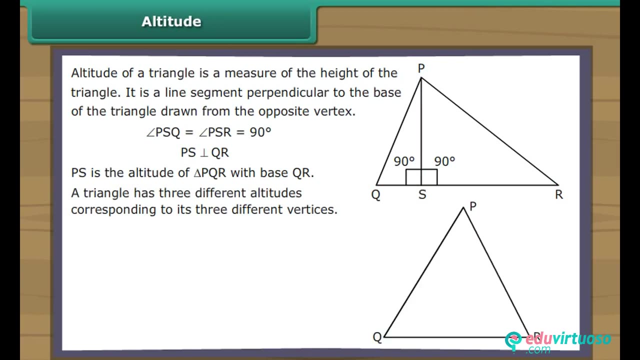 It intersects Q-R at right angles. Therefore, P-S is the altitude of the triangle, P-Q-R with base Q-R. A triangle has three different altitudes corresponding to its three different vertices. Let us now take a look at the remaining altitudes. 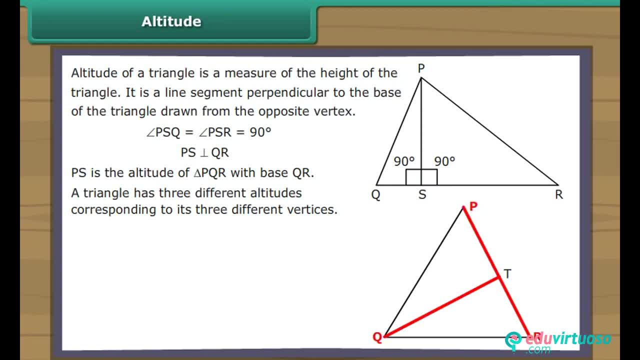 We draw a line segment from Q perpendicular to R-P at point T. It intersects R-P at right angles. Therefore Q-T is the altitude of triangle Q-R-P with base R-P. We draw another line segment from R perpendicular to P-Q at point U. 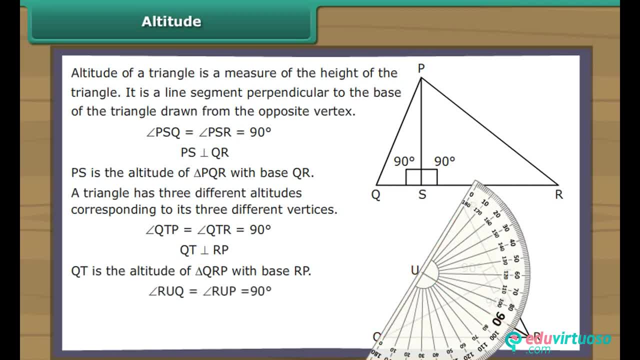 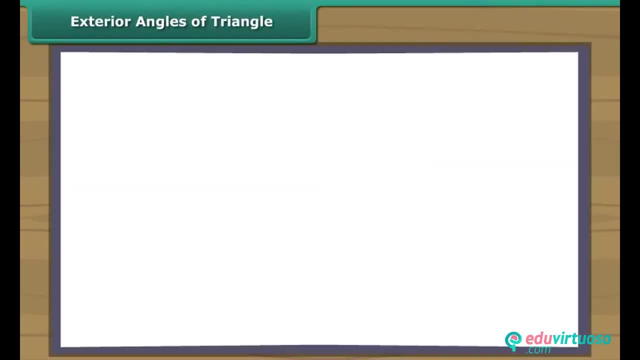 It intersects P-Q at right angles. Therefore, R-U is the altitude of triangle R-P-Q with base P-Q. Exterior angles of triangle. A triangle has three interior angles. It also has some exterior angles. Let us take a look at them now. 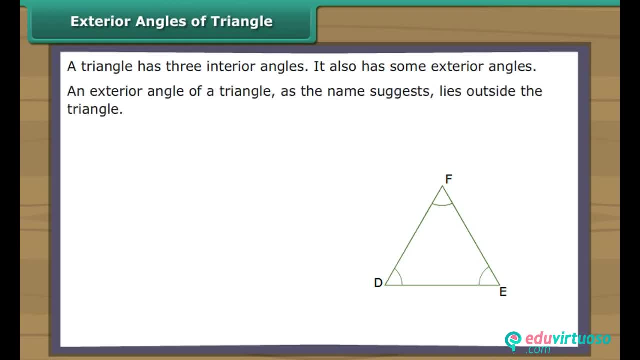 An exterior angle of a triangle, as the name suggests, lies outside the triangle. Exterior angle is formed when we extend a vertex of a triangle. A triangle has six exterior angles corresponding to its three vertices. If we extend vertex E, E of triangle F-D-E, 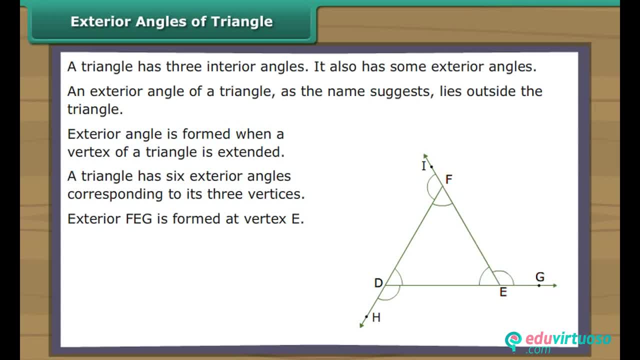 exterior angle F-E-G is formed. Similarly, when we extend the vertices D and F, exterior angles E-D-H and D-F-I are formed. The measure of an exterior angle of a triangle is equal to the sum of the measures of its interior opposite angles. 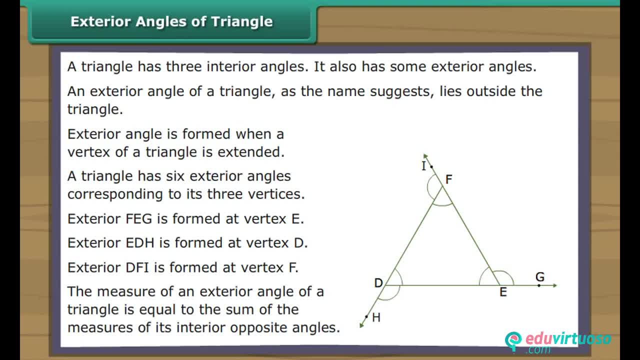 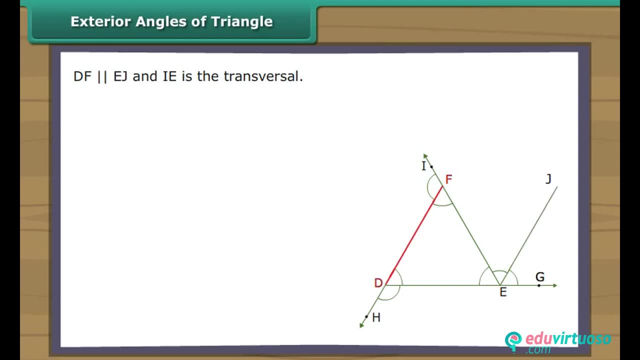 In the figure, angle F-E-G is equal to the sum of angles F-D-E and D-F-E. Let us now prove the same. We draw a line, segment E-J, from point E, such that E-J is parallel to D-F. If we regard I-E as a transversal intersecting the parallel lines. 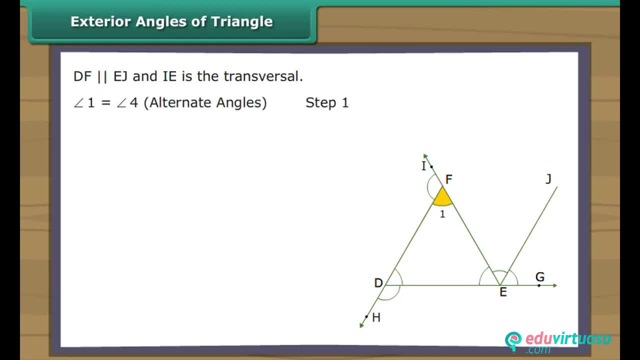 D-F and E-J, angle 1 is equal to angle 4.. Alternate angles: If we regard D-G as a transversal intersecting the parallel lines D-F and E-J, angle 1 is equal to angle 4.. Angle 2 is equal to angle 5.. 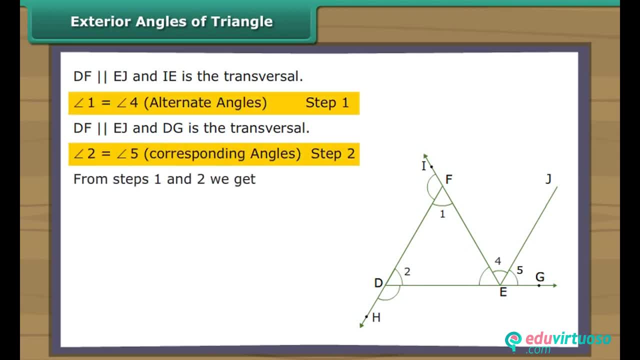 Corresponding angles. From the two steps we get: angle 1 plus angle 2 is equal to angle 4 plus angle 5. It means angle F-E-G is equal to angle D-F-E plus angle F-D-E. Therefore, an exterior angle of a triangle. 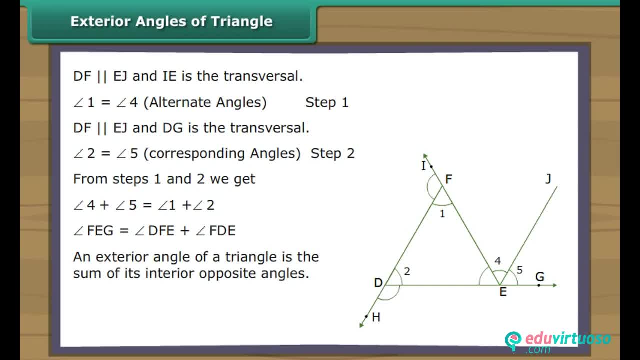 is the sum of its interior opposite angles. Similarly, exterior angle E-D-H is equal to angle D-F-E plus angle D-E-F, and exterior angle D-F-I is equal to angle F-D-E plus angle D-E-F. Self-assessment. 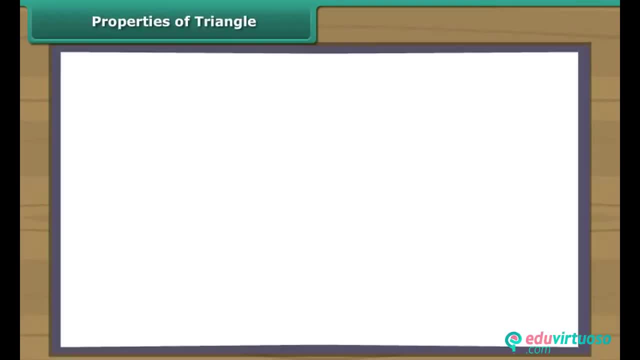 Read the question carefully and select the correct answer. Properties of triangle. The three angles and sides of a triangle exhibit some special properties: Angle sum property. Sum of lengths of sides property. Let us now learn about them one by one. Angle sum property. 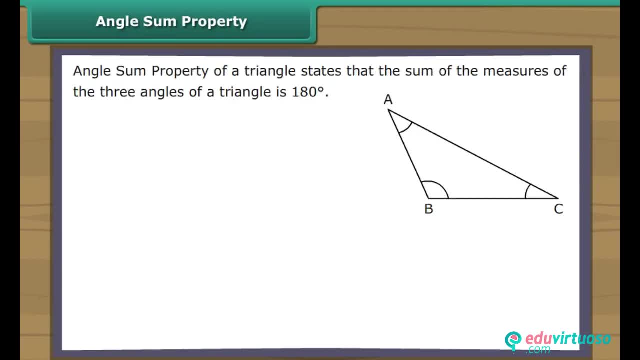 Angle sum property of a triangle states that the sum of the measures of the three angles of a triangle is 180 degree. In the figure, angle A plus angle B plus angle C is equal to 180 degrees. Let us now prove the angle sum property of a triangle. 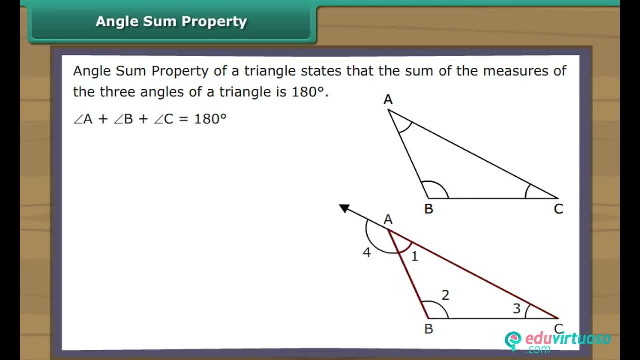 Let us now prove the angle sum property of a triangle. Extend angle BAC Angle 4 is equal to angle 2 plus angle 3 by exterior angle property. Adding angle 1 to both sides we get angle 1 plus angle 4. 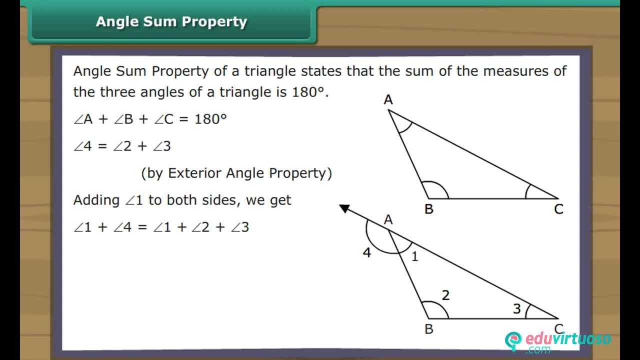 is equal to angle 1 plus angle 2 plus angle 3.. Angle 1 plus angle 4 is equal to 180 degree linear pair. It means angle 1 plus angle 3 is equal to 180 degree linear pair. Angle 1 plus angle 4 is equal to. 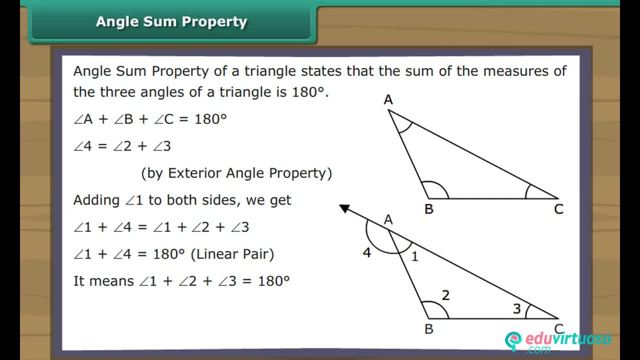 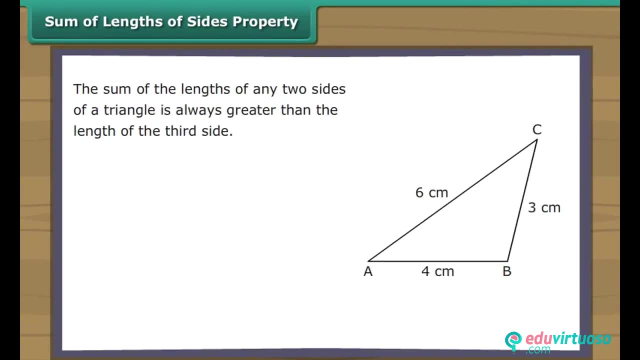 angle 2 plus angle 3 is equal to 180 degrees. Therefore, the sum of the measures of the three angles of a triangle is 180 degrees. Sum of lengths of sides property. The sum of the lengths of any two sides of a triangle is always greater than the length. 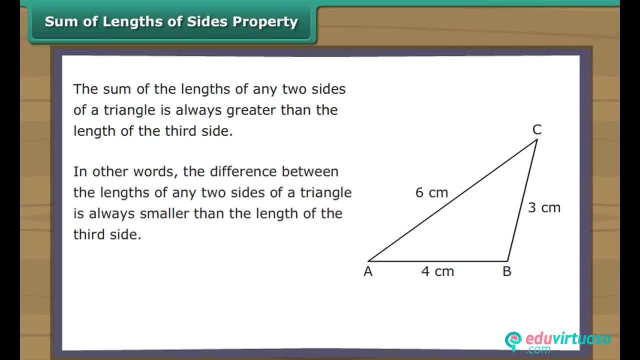 of the third side. In other words, the difference between the lengths of any two sides of a triangle is always smaller than the length of the third side. Three line segments whose lengths do not satisfy this property cannot form a triangle. In the triangle, LMN, LM is 5 cm long, MN is 4 cm long and NL is 7 cm long. 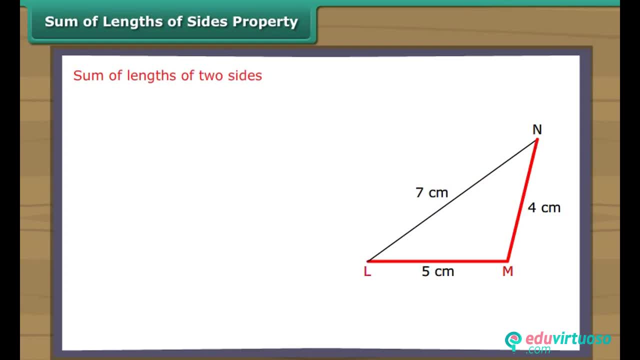 Let us first look at the sum of the lengths of two sides. LM plus MN is equal to 5 plus 4, which equals 9 cm, which is greater than. LM plus MN is equal to 5 plus 4, which equals 9 cm, which is greater than. 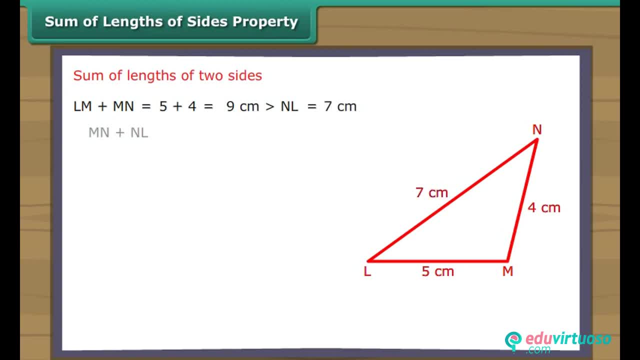 NL, which equals 7 cm. MN plus NL is equal to 4 plus 7, which equals 11 cm, which is greater than LM, which is 5 cm. NL plus LM is equal to 7 plus 5, which equals 12 cm, which is greater than MN, which is 4 cm. 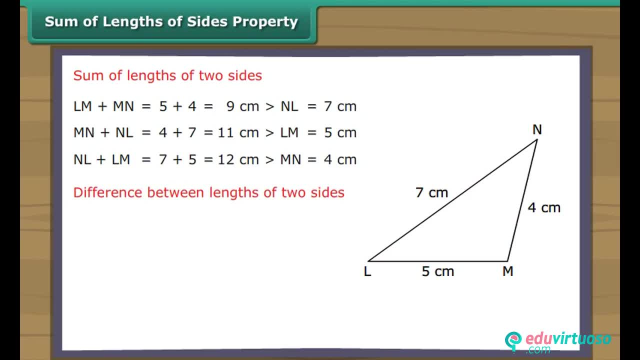 Now let us look at the difference between the lengths of two sides. LM minus MN is equal to 5 minus 4, which equals 1 cm, which is smaller than NL, which is 7 cm. NL minus MN is equal to 7 minus 4, which equals 3 cm, which is smaller than LM, which is 5 cm. 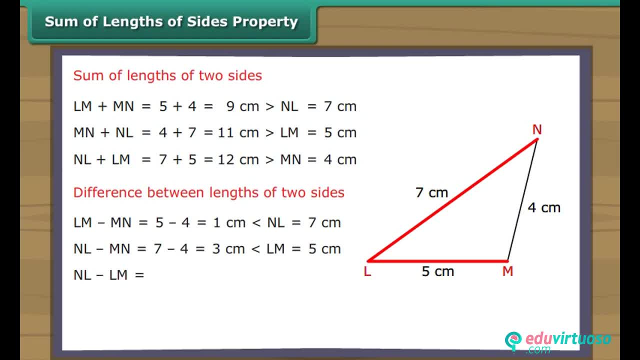 NL minus LM is equal to 7 minus 5, which equals 2 cm, which is smaller than LM, which is 5 cm. Now let us look at the difference between the lengths of two sides than mn, which is 4 centimeter. triangle lmn satisfy the sum of lengths of sites property. 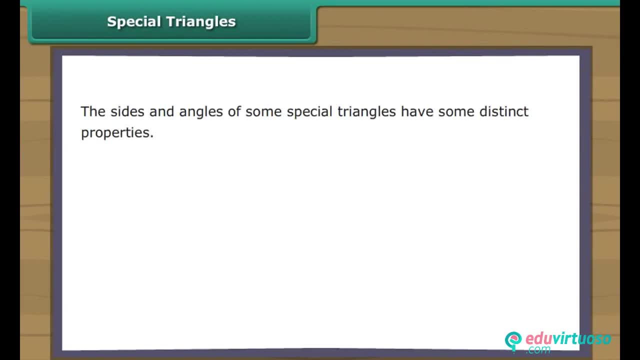 special triangles. the sites and angles of some special triangles have some distinct properties. these special triangles are: equilateral triangle, isosceles triangle, right angled triangle. let us learn about them. equilateral triangle: equilateral triangle is a triangle whose three sites are equal to one another. in triangle, rst, rs is equal to st, which equals tr in an. 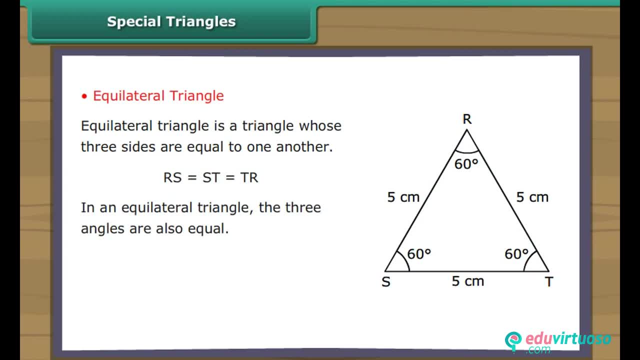 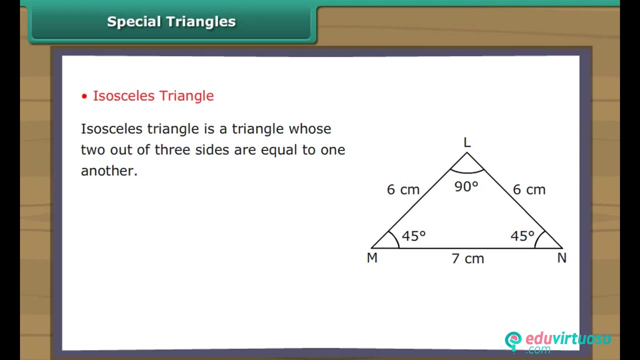 equilateral triangle, the three angles are also equal in triangle rst. angle rst is equal to angle str, which equals angle trs. therefore, an equilateral triangle is also equi-angular isosceles triangle. isosceles triangle is a triangle whose two out of three sites are equal. 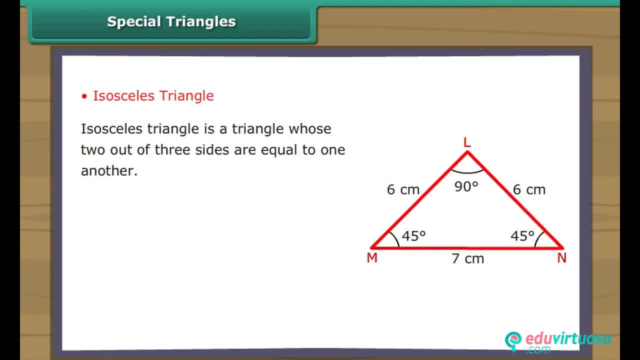 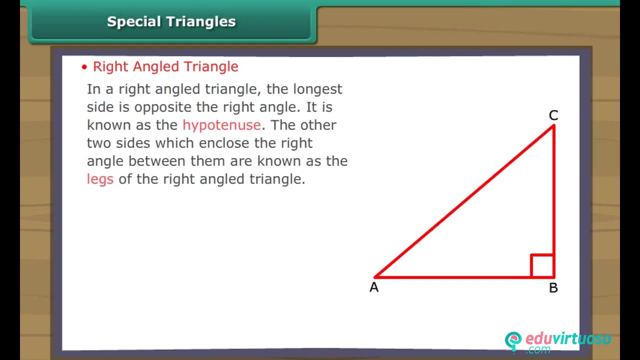 to one another. in triangle lmn, lm is equal to ln. in an isosceles triangle, angles opposite to equal sites are oftentimes equal to angle str. equal. in triangle LMN angle LMN is equal to angle L and M. right angled triangle. in a right angled triangle, the longest side is opposite the right angle. it is: 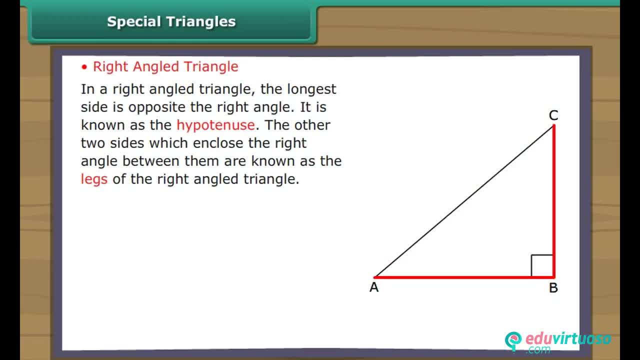 known as the hypotenuse. the two sides which enclose the right angle between them are known as the legs of the right angled triangle, according to Pythagoras, property discovered by a Greek philosopher by the name Pythagoras. sum of squares of lengths of two legs of a right angled triangle is equal to the 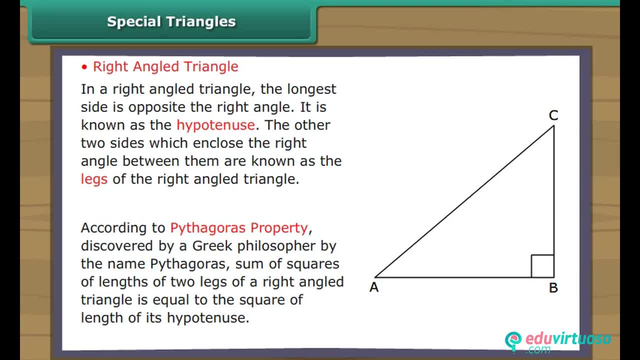 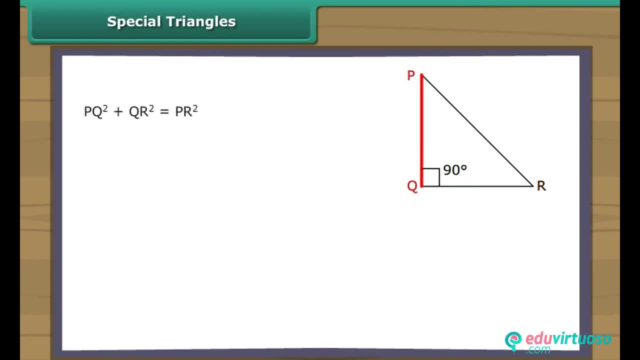 square of length of its hypotenuse. according to Pythagoras property, in right angled triangle PQ are: PQ square plus QR square is equal to PR square. in triangle XYZ, it is given that XY square plus y z square is equal to X Z square. let us measure angle x, y, Z of.